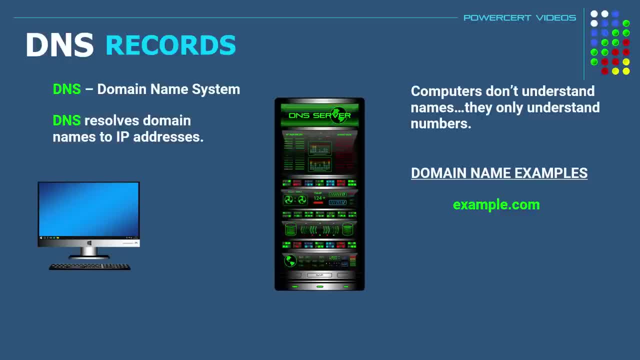 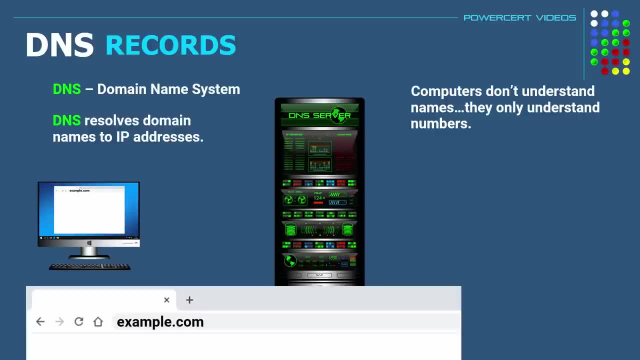 when you want to go to a certain website, such as examplecom, googlecom, yahoocom and so on. So when you type in a domain name such as examplecom in a web browser, DNS will resolve that domain name into an IP address so you can retrieve the web address. 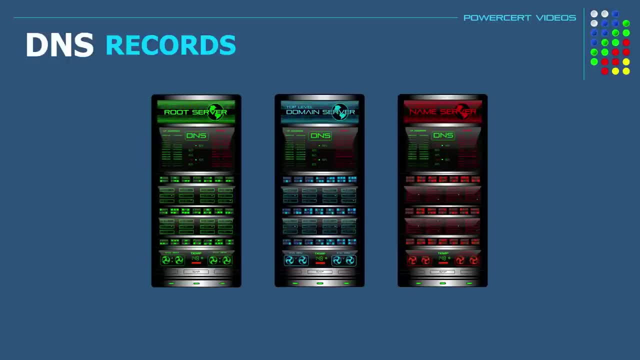 Now, in a DNS hierarchy, there are three main levels of servers. There are the root servers, the top level domain servers and the authoritative name servers. But of these three, the DNS servers that are responsible for storing the DNS records for resolving domain names to IP. 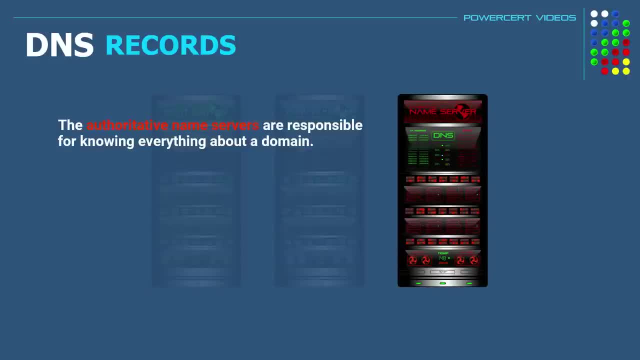 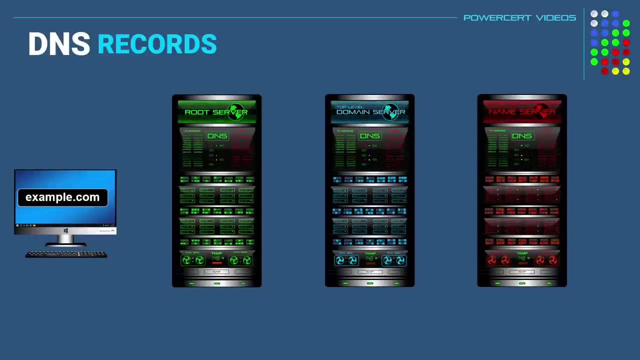 addresses are the authoritative name servers because they are responsible for knowing everything about the domain name, including the IP addresses and the domain names. But in order for your query to resolve examplecom into an IP address, it needs to know which name server to ask. So in order to find the correct name server, the query must first go through the. 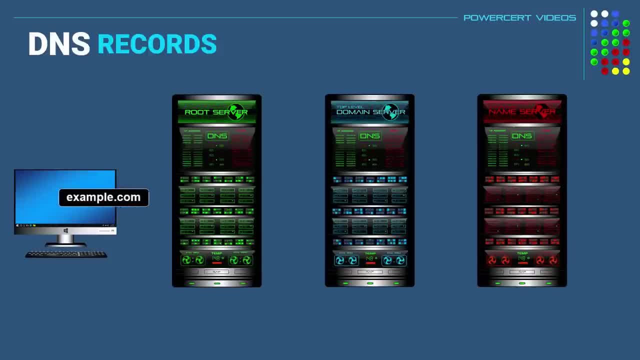 top of the DNS hierarchy, which is the root server, And once it reaches the root server, the root server will look at examplecom and will forward the query to the correct top level domain server. The top level domain server is responsible for information of the top-level domains, such as com, net, org and so on. So in 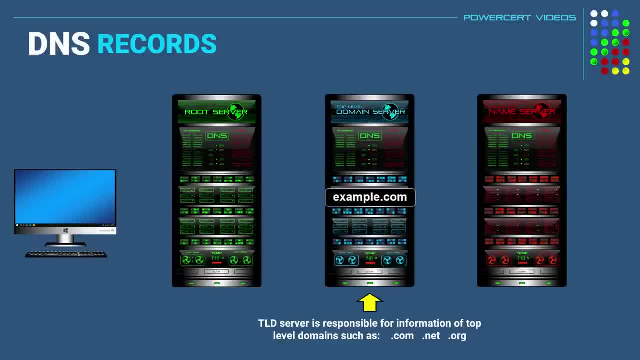 this case, the root server will forward the query to the com top-level domain server, because the top-level domain for examplecom is com, And then the top-level domain server will forward the query to the specific authoritative name server that's responsible for the examplecom domain And once. 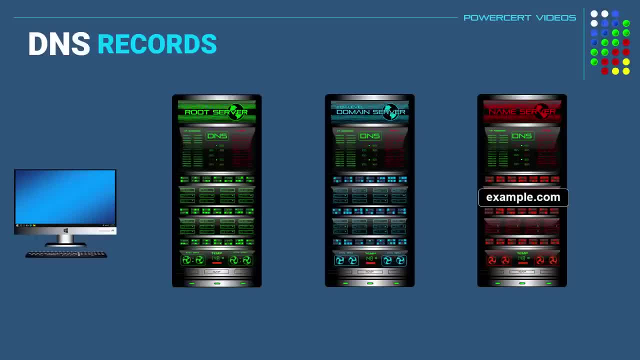 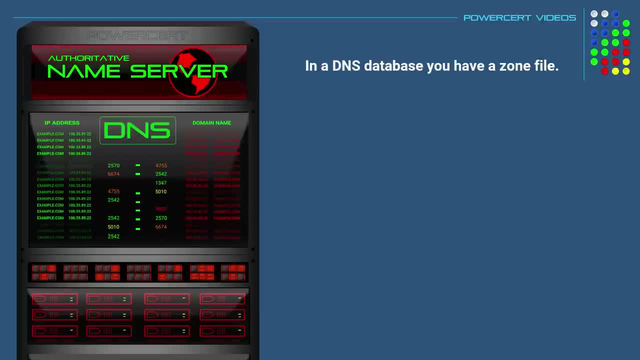 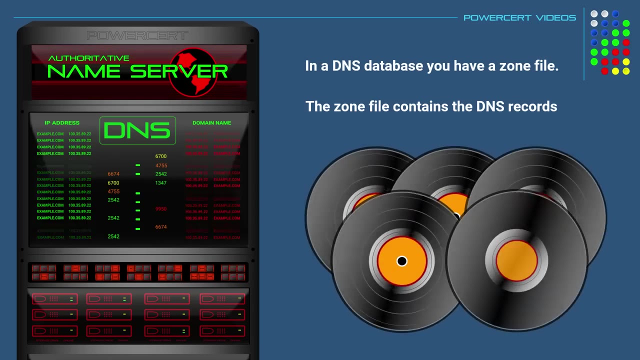 the query reaches the name server examplecom, will be resolved to the IP address, so the website can be retrieved. So in a DNS database you have what's called a DNS zone file and this file contains the DNS records. Now there are numerous DNS records, but I'm only going to talk about the most common. 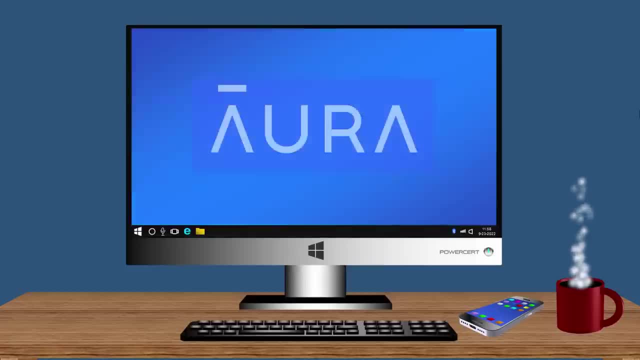 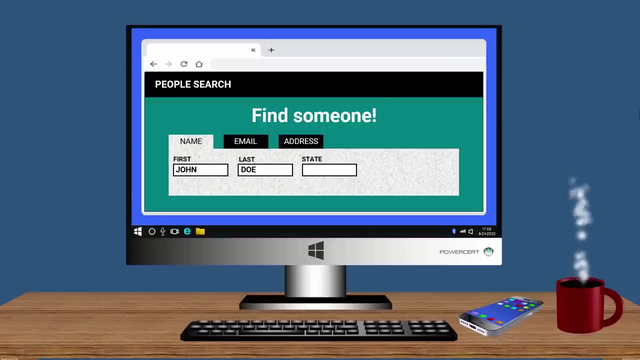 ones. Hey guys, I just want to break in this video and tell you about my partnership with Aura. Now, anyone can find anything on the internet, including the Aura database. Now I'm going to talk about the Aura database. So I'm going to talk about the Aura database Now. Aura is the database that 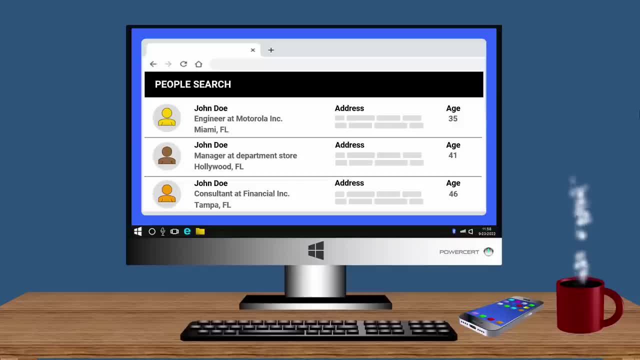 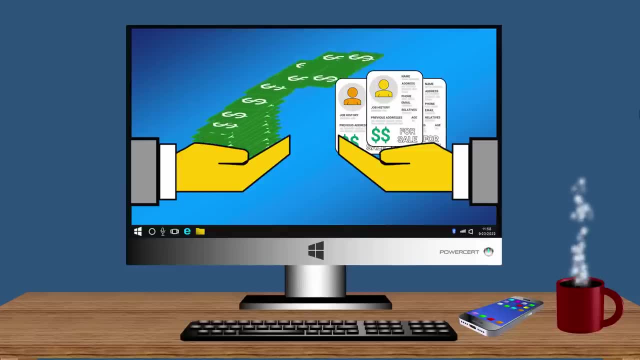 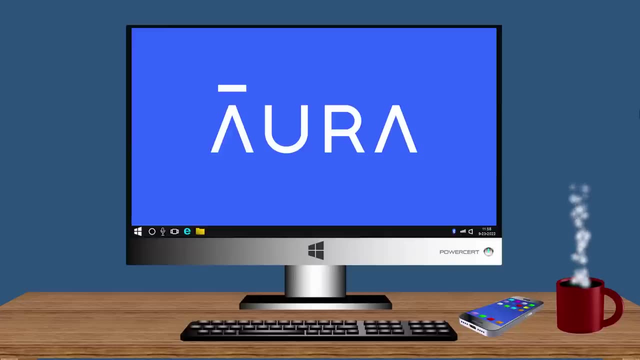 has access to all your files, including your full legal name, your personal email, home address, phone number and even your relatives. Now this information is accessible because of data brokers who profit by selling your information to robocallers, telemarketers, spammers and anyone. 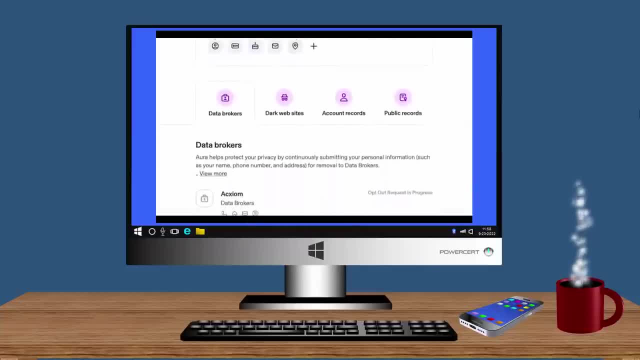 else that wants to learn more about you, So that's why I want to tell you about my partnership with Aura. Aura will identify brokers that are exposing your information and automatically submit opt-out. time I used Aura, I was surprised to see that over 20 data brokers had information about me and Aura. 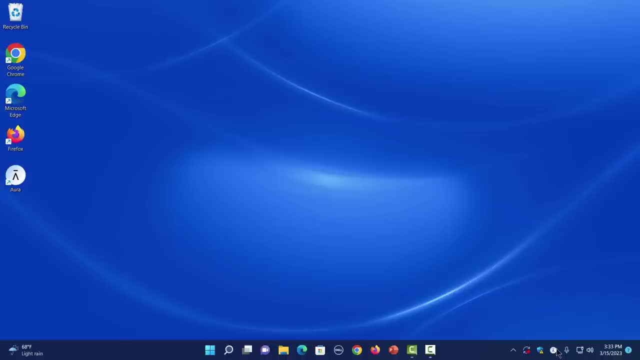 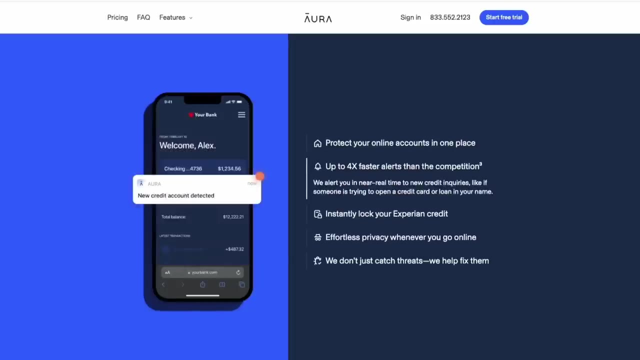 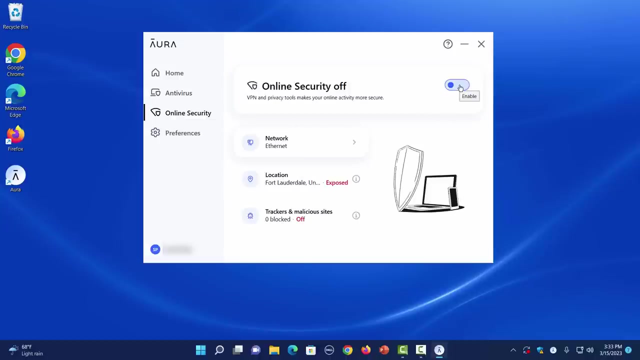 quickly went to work to remove that information. Aura also has an app that features an antivirus password manager and real-time credit and identity theft monitoring that will alert you if there's a credit inquiry in your name, And I know a lot of my viewers are going to like this. but the app even 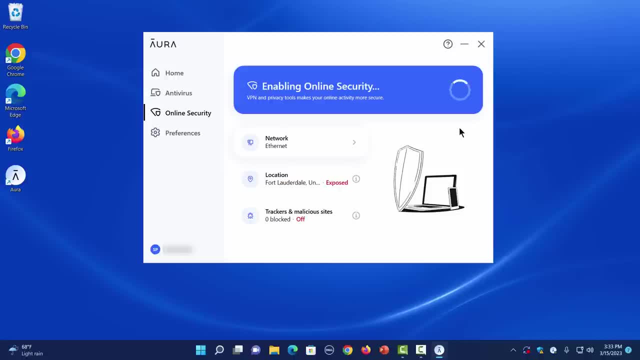 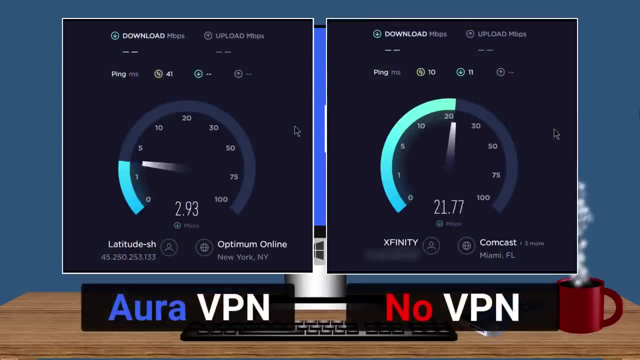 has a super fast built-in VPN, so you can serve the internet safely and anonymously. In fact, the VPN is so fast that there's hardly any difference when I did a speed test on my computer- and you can see the speed test results here- with and without using Aura's VPN. So Aura has almost every internet. 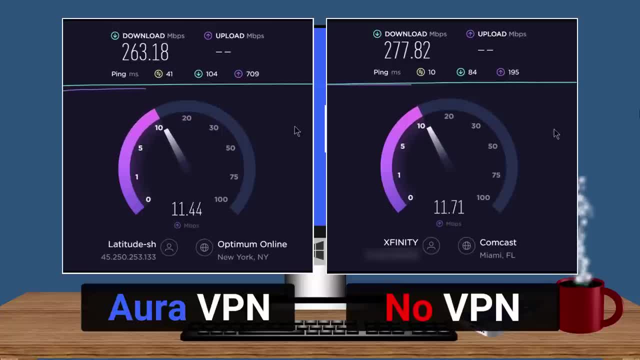 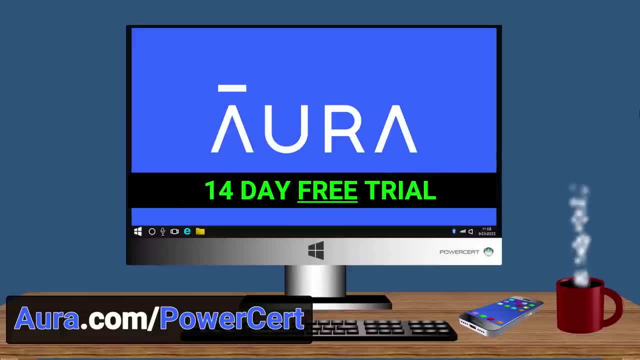 safety tool you'll ever need, all inside one app. And if you sign up right now, they will give you a two-week free trial and you'll be shocked of how much your private information Aura finds exposed over those two weeks. So just go to Auracom forward slash power cert, which will be 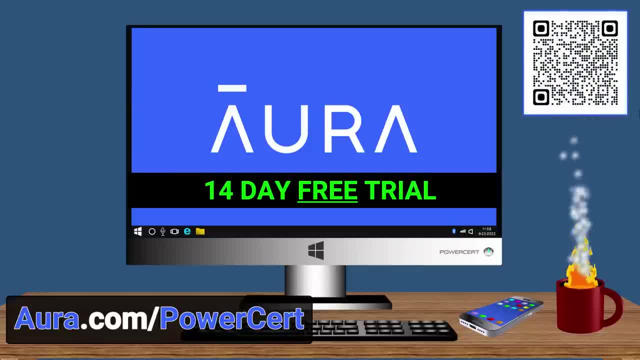 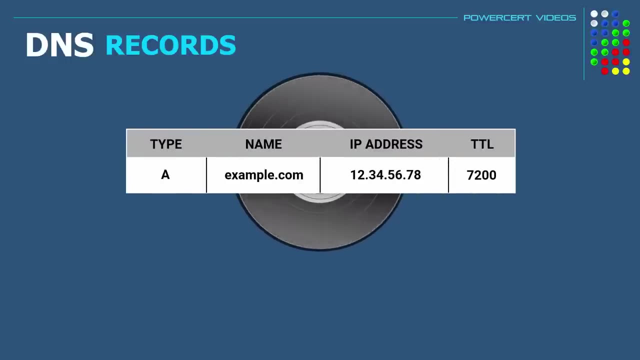 in the link in the description below, or you can scan the QR code on the screen to try two weeks for free and see for yourself how many data brokers are sharing your personal information. So the first DNS record is the A record or address record, and this is the most common DNS record. 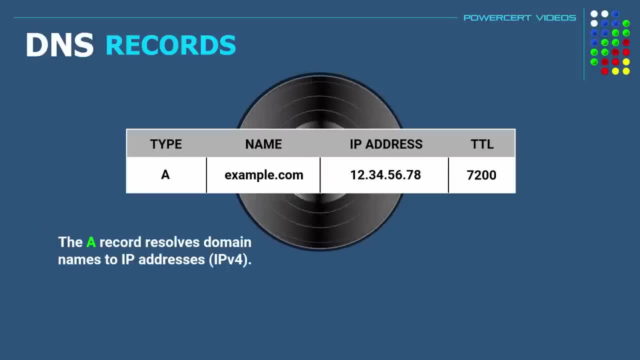 This is what resolves a domain name to an IP address. To be sure, you need to have a domain name and a IP address. To be specific, it resolves to an IP version 4 address, which is a 32-bit numeric address. So in the example we just did earlier, when you type in a domain name such as examplecom, in a 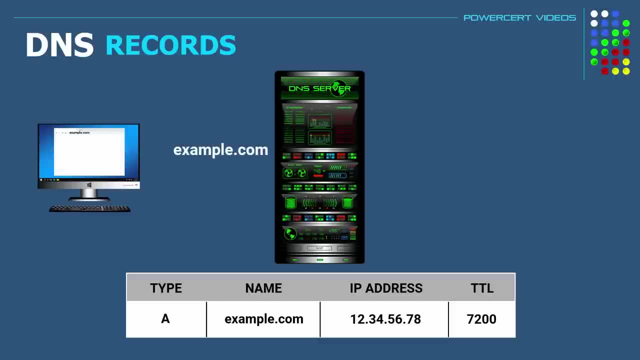 web browser. the A record is what DNS uses to resolve a domain name to an IP address. And then we also have the TTL, or time to live. This field tells us how long each record is valid until the next update. And then there's also the 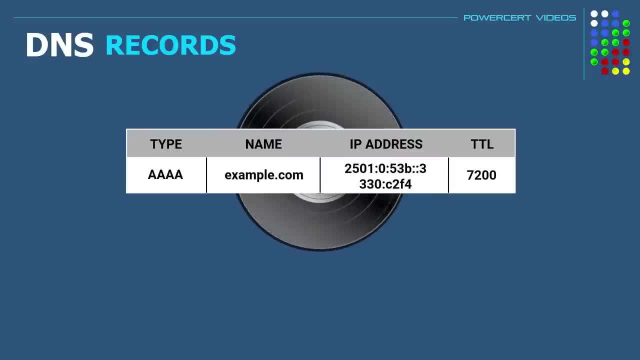 quad A record And this record is just like the A record. So both A and quad A records resolve domain names to IP addresses. But the difference is is that quad A records resolve domain names to IP version 6 addresses. An IP version 6 address is a 128-bit alphanumeric address that's replacing 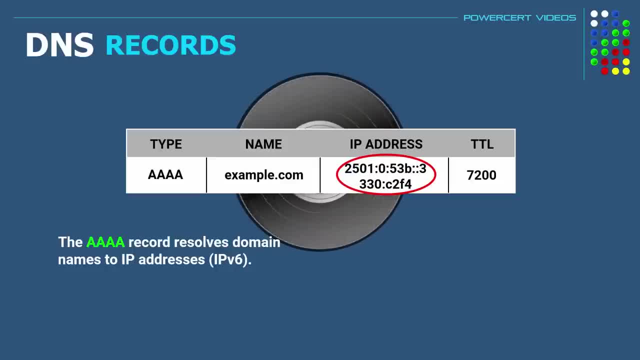 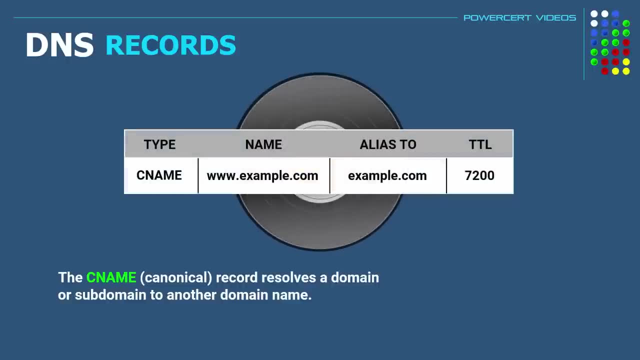 the older IP, version 4, addresses. The next DNS record is called CNAME or canonical name, And what this does is that it resolves a domain or subdomain to another domain name. So basically it's an alias for another domain name. So, as an example, computers read domain names from right. 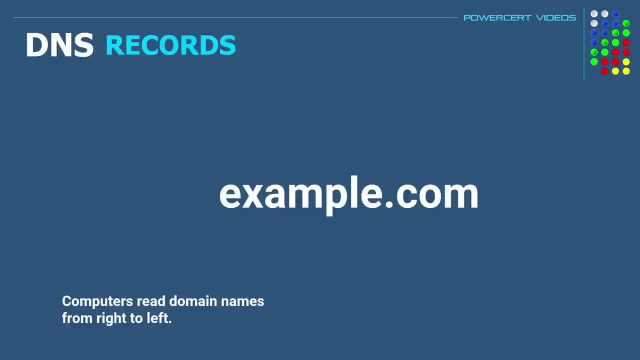 to left And domain names will have several parts: A root domain, a top level domain, a second level domain and a subdomain. So when we look at examplecom, there is also a hidden dot right after com, Even though it's hidden and we don't see it. but that dot is the root domain, The dot com is the 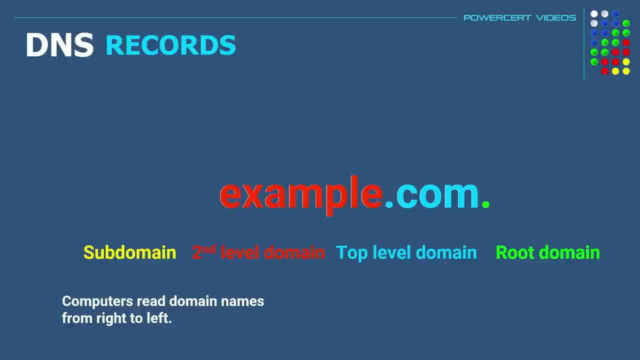 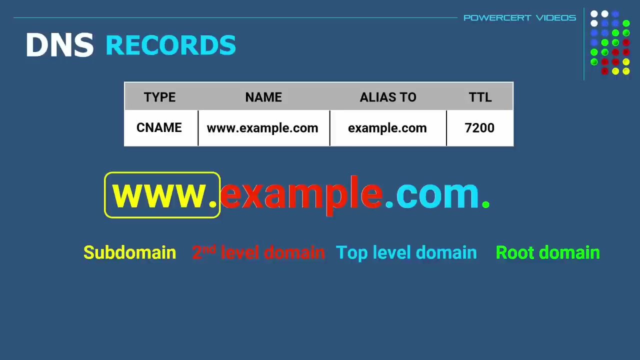 top level domain And example is the second level domain. But if there is an additional name to the left of a second level domain, then that would be a subdomain. So, for example, www is a common subdomain, Which is why it is common to create a CNAME record pointing wwwexamplecom. 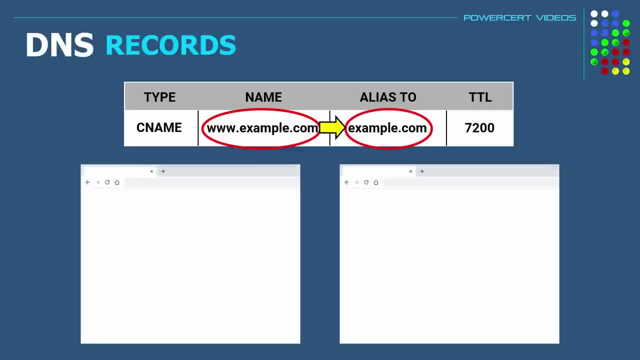 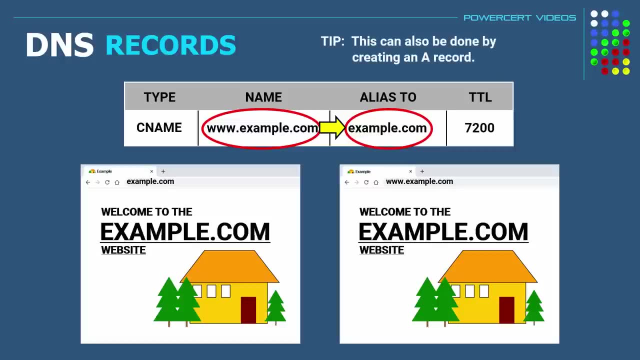 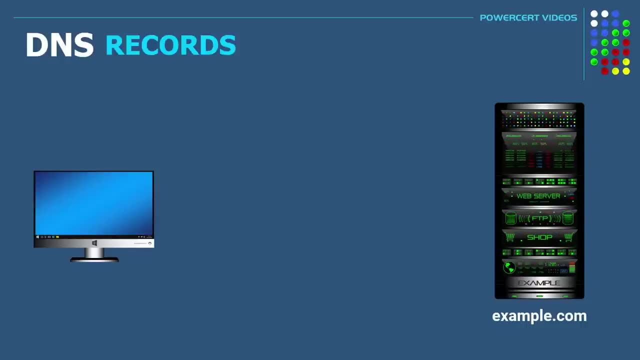 to examplecom, Which is why, when you type examplecom or wwwexamplecom in your web browser, you'll end up at the same examplecom website. because of that CNAME record, Subdomains are also often used when a website has different services running on the same server. 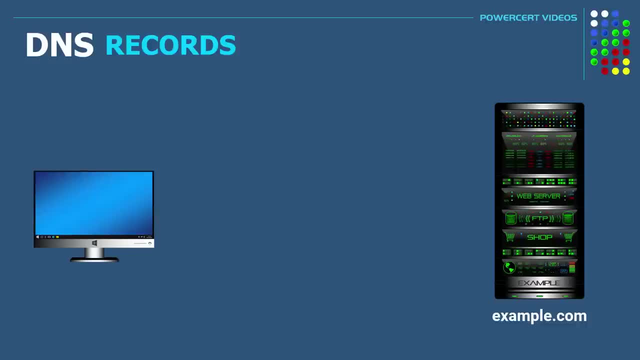 and are using the same IP address. So, as an example, let's say that examplecom has an FTP service running on the ad fork. That could be an example or whatever you're using, And the examplecom you want an example gets an here and now example, and then the examplecom you want 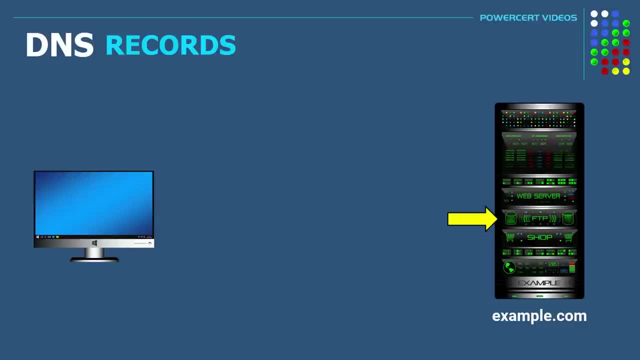 on the same server as their website. So in this case they can create a subdomain, such as ftpexamplecom, for their FTP service on the server, And then they can create a CNAME record and have it directed to examplecom. So now when users type in ftpexamplecom in their web browser, 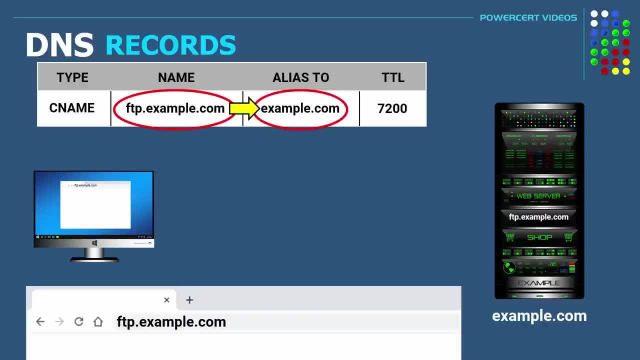 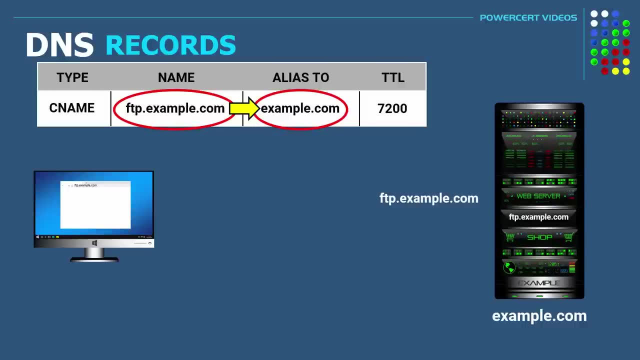 DNS will look at the CNAME record and forward the users to examplecom Now, even though it's pointing to examplecom. but once the request reaches the web server, the web server will inspect the URL that the user has typed and direct it to its FTP service on the server. So CNAME records. 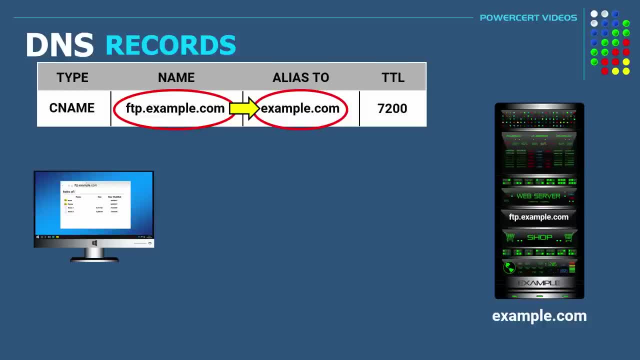 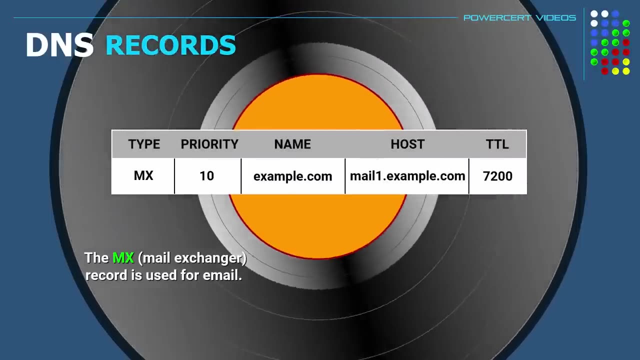 are similar to A records, but the difference is is that A records resolve domain names to IP addresses, while CNAME resolve domain names to domain names. And the next DNS record is MX record or mail exchanger record, And this record is used for email. The MX record simply points to the. 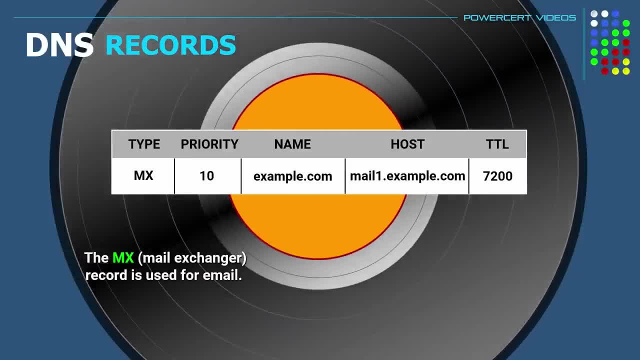 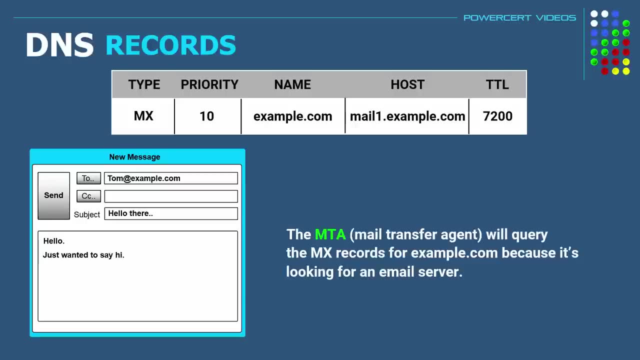 server where email should be delivered for that domain name. So, for example, when you send an email to tom at examplecom, your MTA or mail transfer agent will query the MX records for examplecom because it's looking for an email server And then DNS will respond back telling. 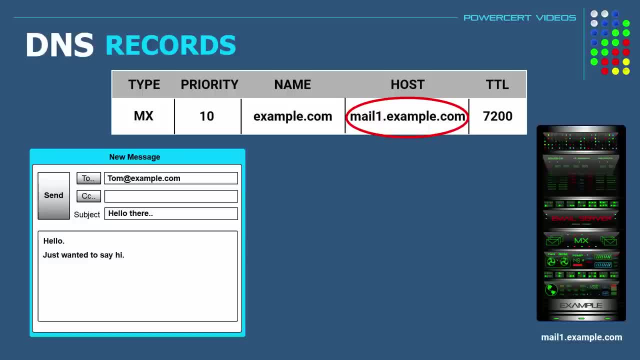 the MTA, which server to send the email to. So go to examplecom and what you will need to do is please fill in the, For example, mta or mail, and then you need to fill in the, For example, which server. 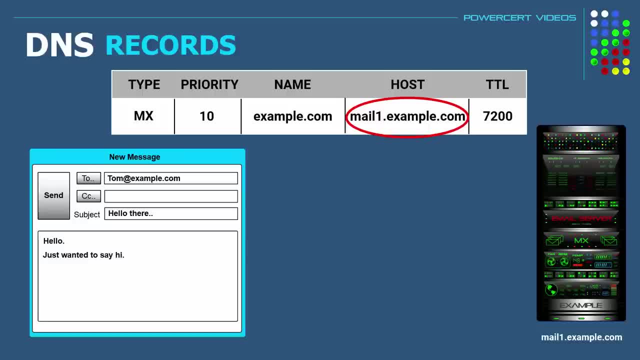 will ask you to use when sending a mail exchange And what and when, And the answer is either to send an email request or only when terms betweenapr, where the email is generated, and that the e-mail recovery, Which in this case would be mail1.examplecom. 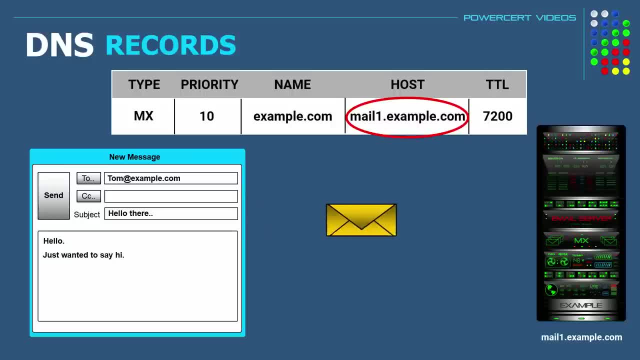 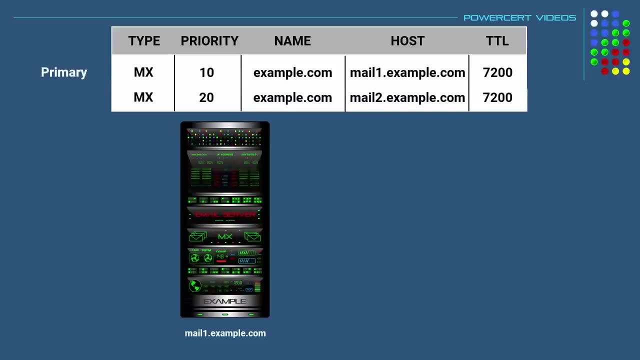 Because that's what the MX record points to. So that's basically what the MX record does: It tells the world which server to send email to for a particular domain name. Now, MX records will generally have two entries: A primary email server and a secondary email server. 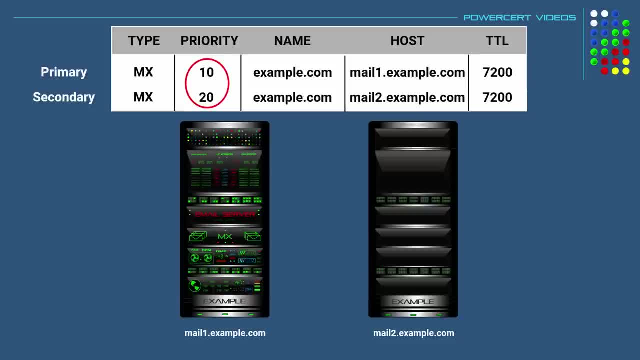 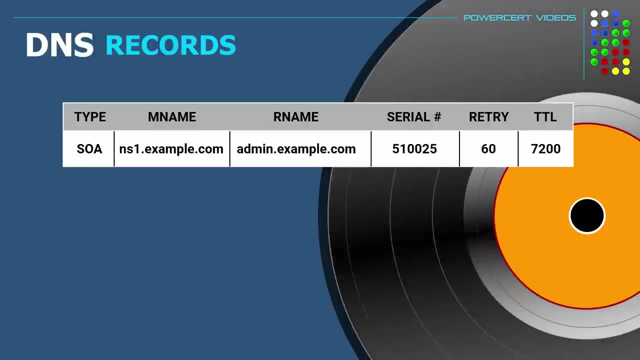 Along with priority numbers, The lower. the priority number means that it's the primary email server, But if the primary email server gets overwhelmed or goes down, then the secondary email server would be used. And the next DNS record is called SOA, which stands for start of authority. 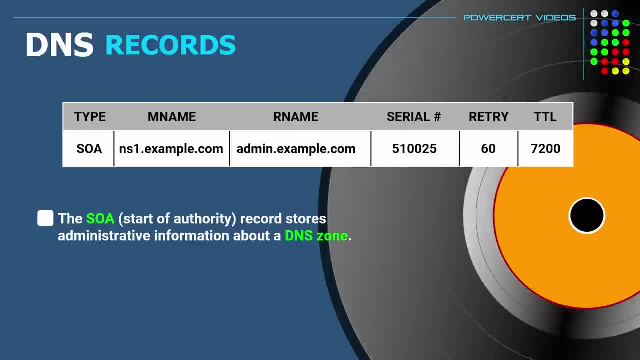 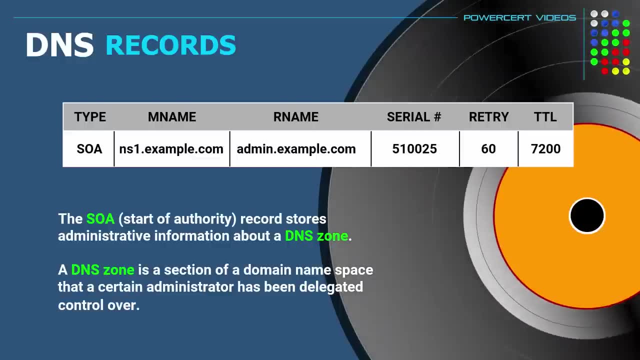 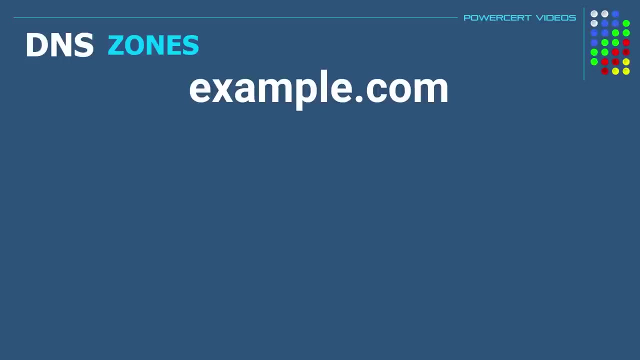 And what this does is that it stores administrative information about a DNS zone. So what are DNS zones? Well, a DNS zone is a section of a domain namespace That a certain administrator has been delegated. control over DNS zones allow a domain namespace, such as examplecom, to be divided into different sections. 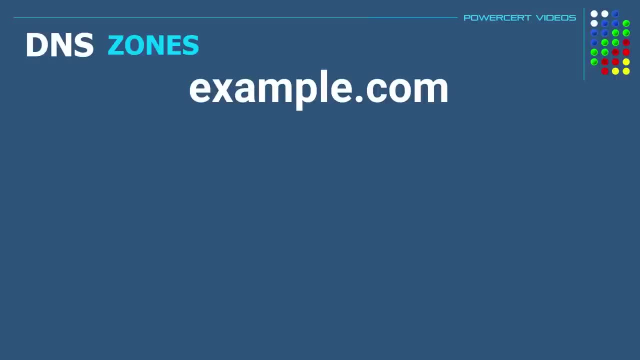 So, if we look at the domain examplecom, If this domain was broken down into three sections or subdomains, Such as shopexamplecom, blogexamplecom and supportexamplecom, The head administrator could create DNS zones And delegate control over these domains. 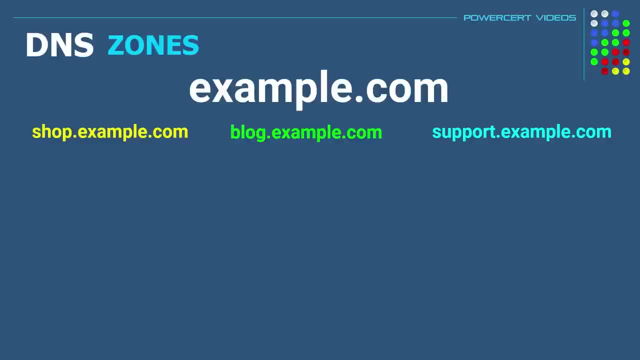 So if we look at the domain examplecom, If this domain was broken down into three sections or subdomains, The head administrator could create DNS zones for these subdomains to different administrators if he chooses to. So let's say that the shop and blog subdomains have only a few computers in each domain. 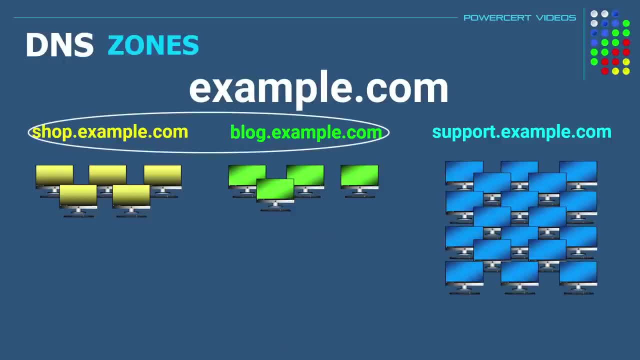 And the support subdomain has many computers. So since these two only have a small amount of computers, the head admin could create one zone for these two subdomains And assign an administrator to manage it. But since support has so many computers, the head administrator has created another separate. 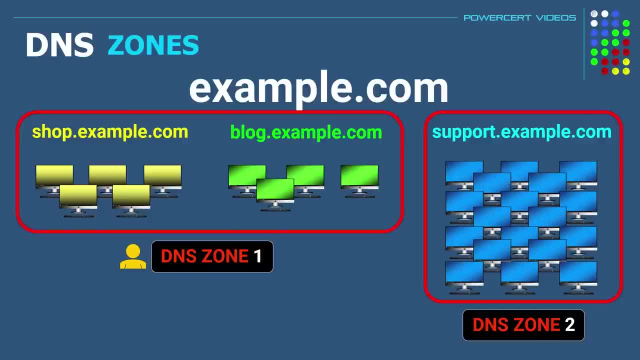 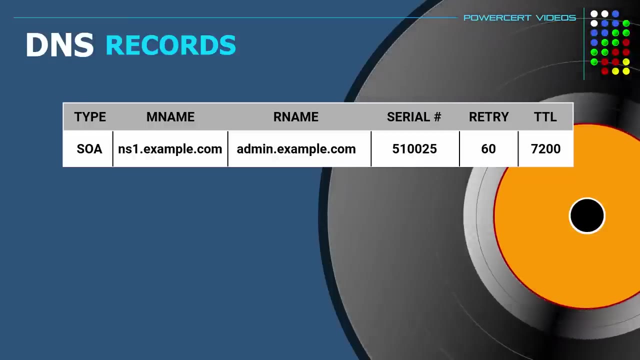 zone, the support subdomain, and then he or she will assign another administrator to manage it. So DNS zones are created for manageability purposes and each will have their own DNS zone file which contains an SOA record. So here is an example of an SOA record. 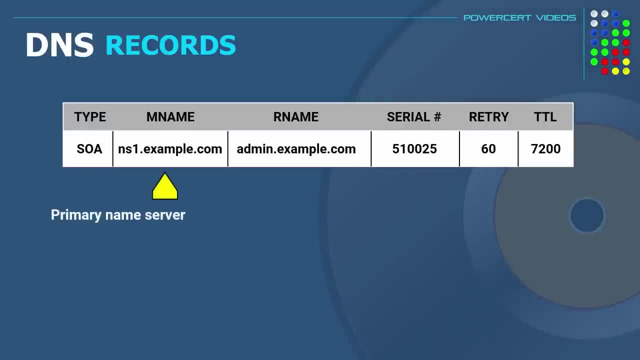 So just to go over a few of these categories, the mname is the primary name server, The rname is the email address of the administrator for this zone, where this dot here represents the at symbol in an email And the serial number is a number that represents a version in the zone. 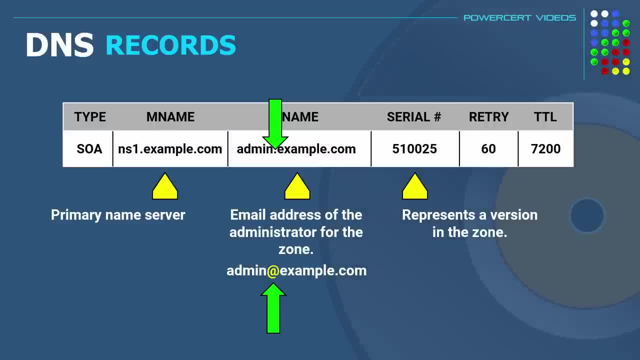 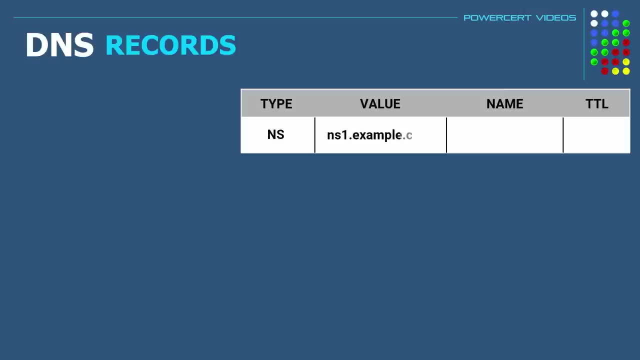 so whenever an update happens in the zone, the serial number will change, which tells the secondary servers to update as well. And the next record is the NS record, which stands for name server. Now this record, just like its name says, provides the name of the authority in some of the different types of the server. 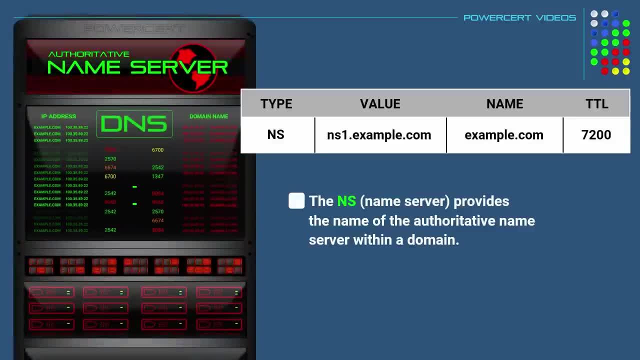 So, for example, if there is a server that uses the name of a server and we get a standalone version authoritative name server within a domain. So, as I stated previously, the name server contains all the DNS records necessary for users to find a computer or server on a local network or on the Internet. 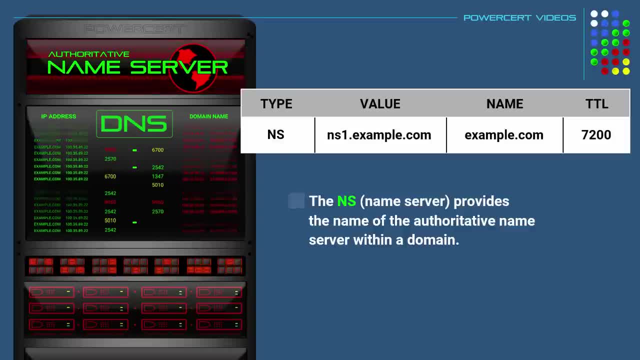 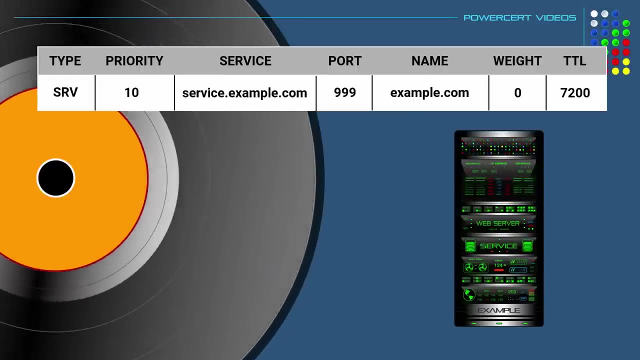 It is the final authority in a DNS hierarchy, and an NS record would generally list two name servers, a primary and a secondary, And the next DNS record is called SRV, which stands for service record. Now, the previous DNS records that we talked about will point to a server or an IP address. 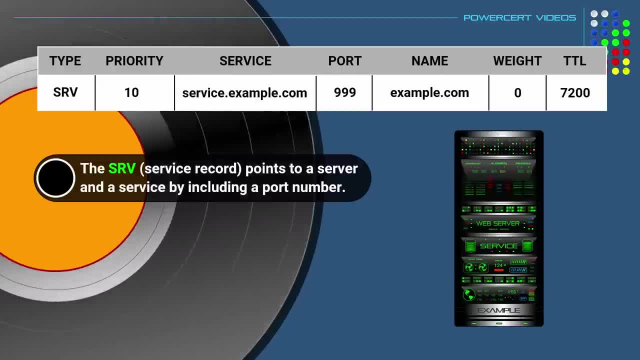 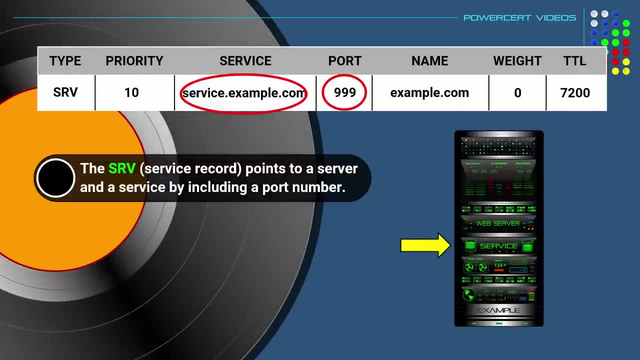 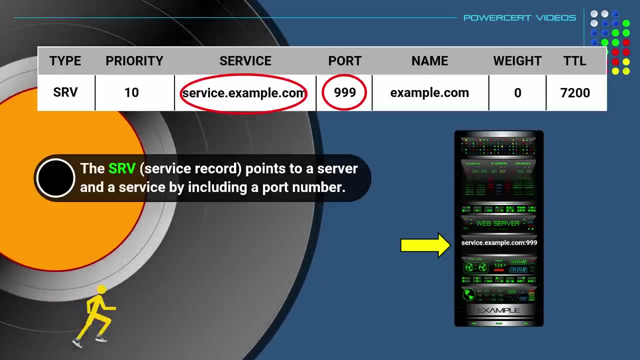 but a service record will point to a server and it'll also point to a specific service by including a port number. So when an application needs to find the location of a service on a domain, such as voice over, IP, instant messaging or a printer, it will look for a service record to see if there's a listing for that specific service and it. 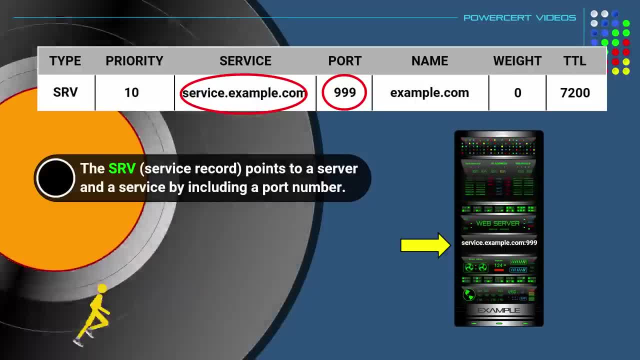 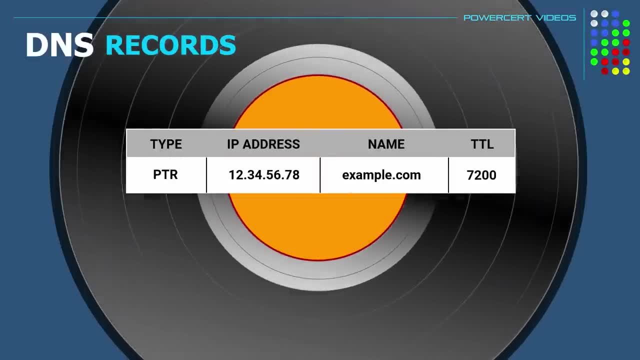 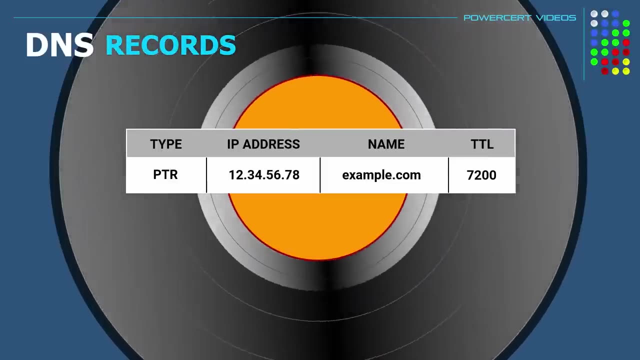 will direct it to the correct server and correct port number, And then we have a PTR or pointer record. Now this record is basically the reverse of an A or a Quad A record. So, as you remember, A and Quad A records resolve domain names to IP addresses. 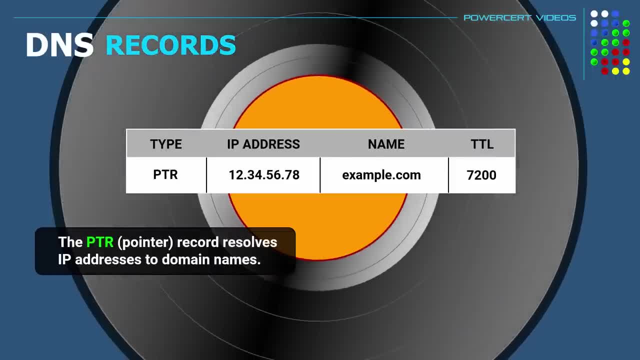 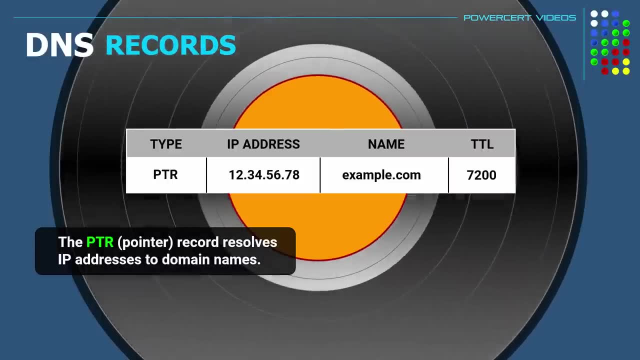 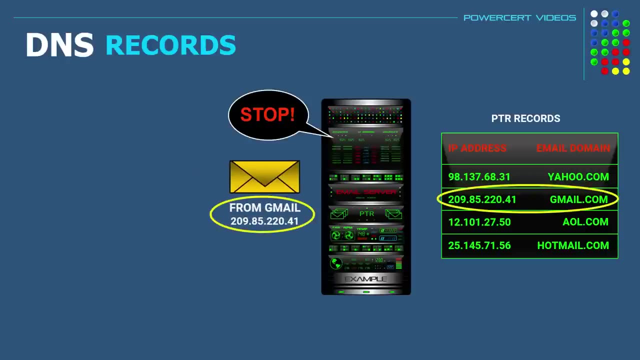 But PTR records do the opposite. They resolve IP addresses to domain names. PTR records are attached to email and are used to prevent email spam. So whenever an email is received, the email server uses the PTR record to make sure that the sender is authentic by matching the domain name in the email with its 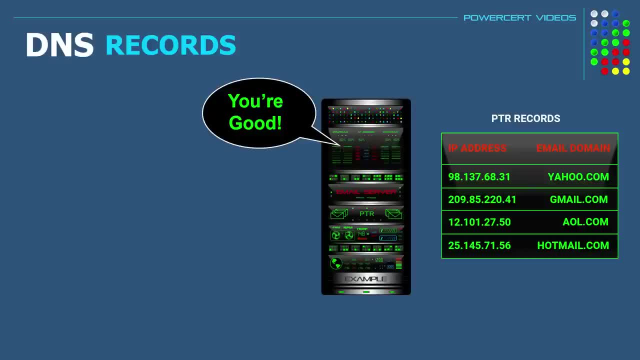 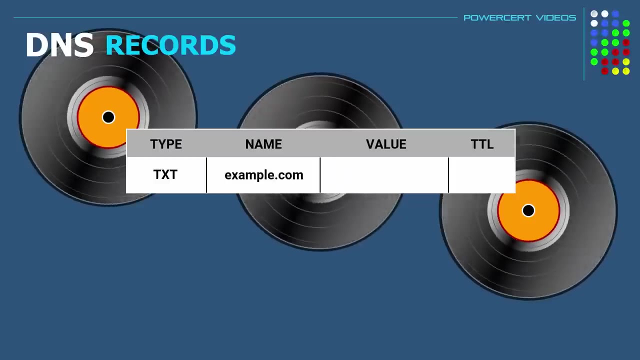 authentic IP address. This is what's known as a reverse DNS lookup. But if an email that is sent does not match with its correct and authentic IP address, the email will be flagged as spam And our last record is the TXT or text. Now, this record contains miscellaneous information about a domain. 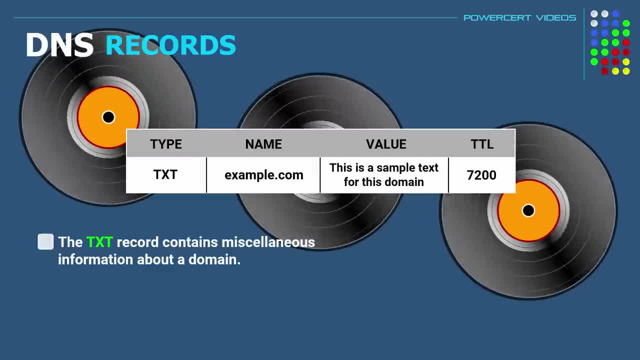 Such as general or contact information. These are also used to prevent email spam by making sure incoming email is coming from a trusted or authorized source. They can also contain other miscellaneous text, such as: be sure you sign up for Aura's two-week free trial at. 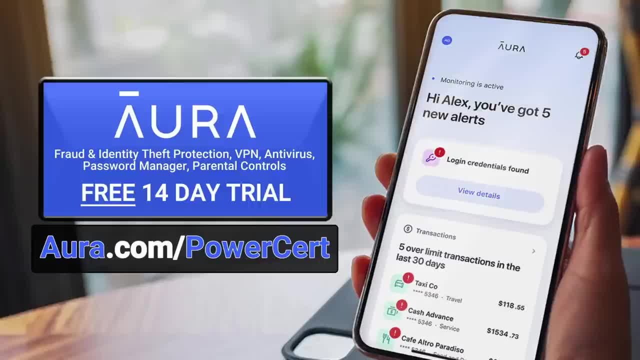 Auracom forward slash power cert. So, guys, I want to thank you for watching this video. please subscribe and I will see you in the next video. You